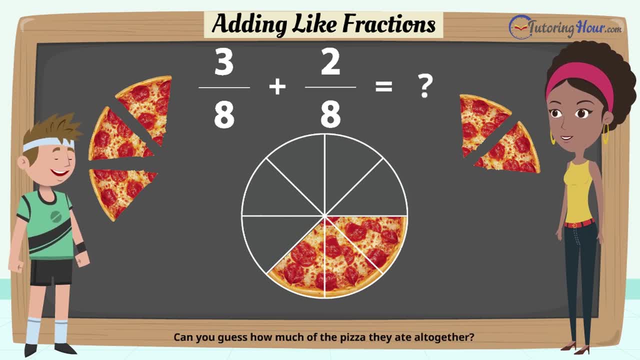 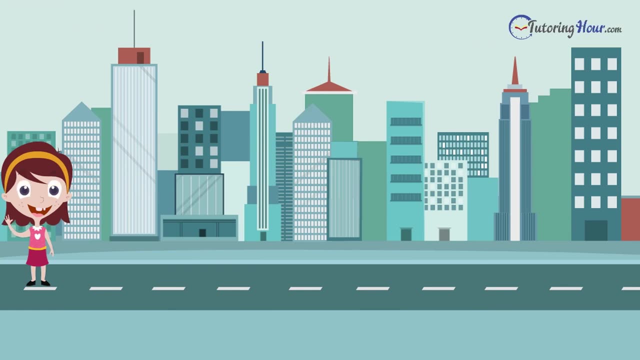 Can you guess how much of the pizza they ate altogether? Yes, you are right, Jake and Amanda ate five out of the eight slices, or five-eighths of the pizza altogether. Yippee, We've got the answer. Let's take another example. Linda walked four-ninths of a mile to reach the library and another three-ninths of a mile to reach the park. 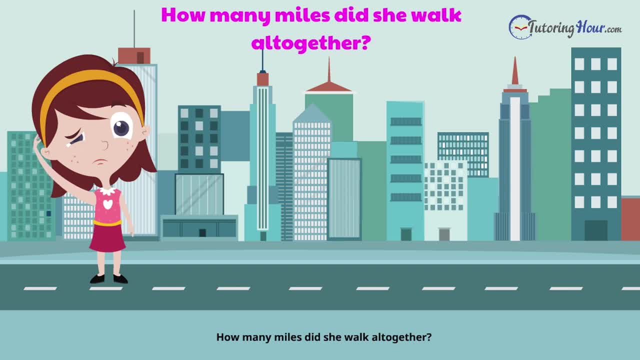 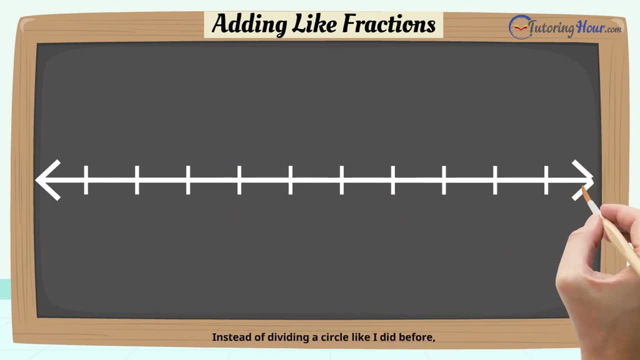 How many miles did she walk altogether? Let me show you an easy way to do it. This time I'll draw a number line. Instead of dividing a circle, like I did before, I'll divide the number line into nine equal parts between zero and one. 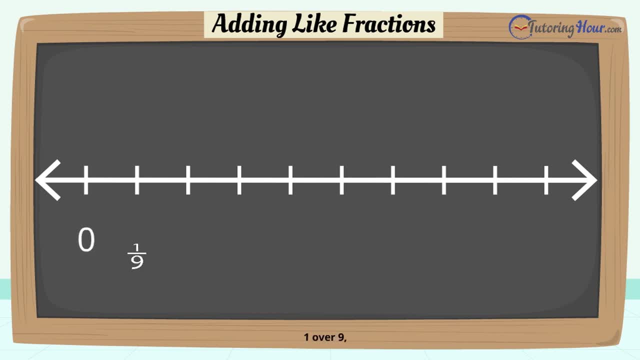 And I'll mark them 0,, 1 over 9,, 2 over 9, and go on until 9 over 9, which becomes a whole. I'll write that as 1.. Now let's move on to the next step. 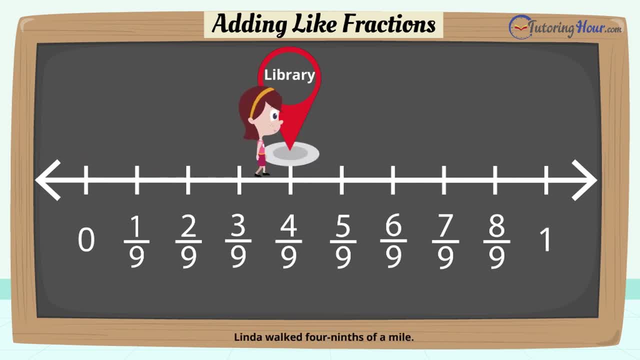 Linda walked four-ninths of a mile, so let's draw a hop from zero to four over 9.. And then she walked another three-ninths of a mile, Starting at four over 9,. I'll draw three more hops covering one-ninth, then two-ninths, then two-ninths. 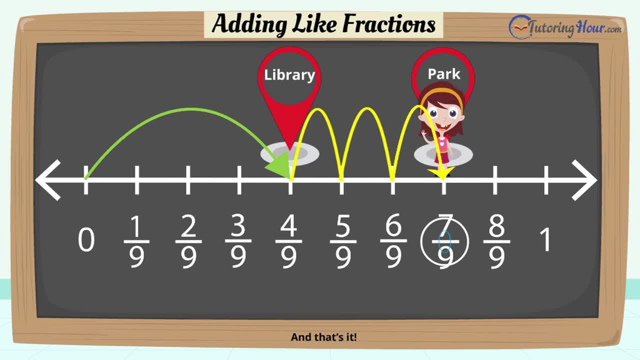 and then 3 9ths of a mile, And that's it. Linda walked 7 9ths of a mile in all. Let's represent this number line model as a fraction addition equation: 4 over 9 plus 3 over. 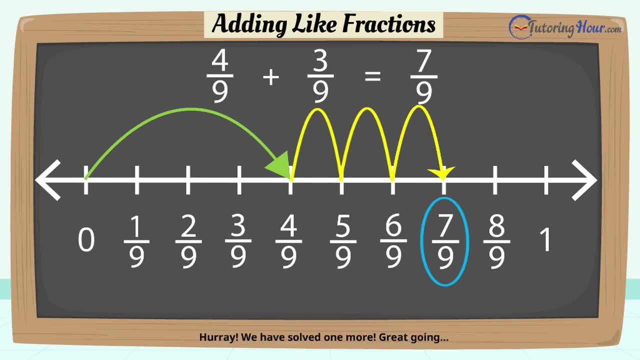 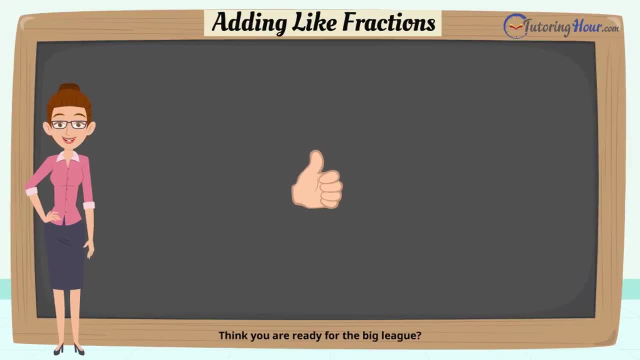 9 makes 7 over 9.. Hooray, We have solved one more Great going. Thank you already for the big leak. Then let's try another problem: 5 over 13 plus 7 over 13.. Look at both these fractions They have. 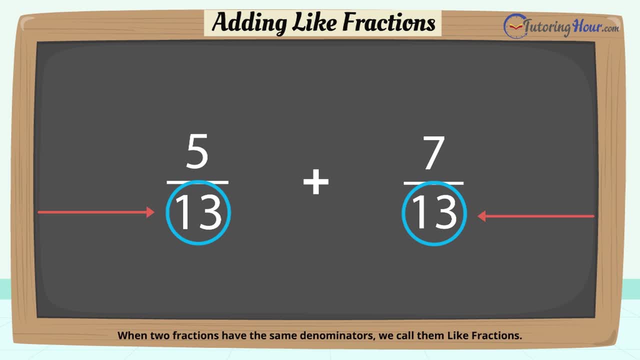 the same denominators. When two fractions have the same denominators, we call them like fractions. While adding like fractions, we don't add the denominators, We simply retain them. We only add the top numbers and write the sum over the common denominator. 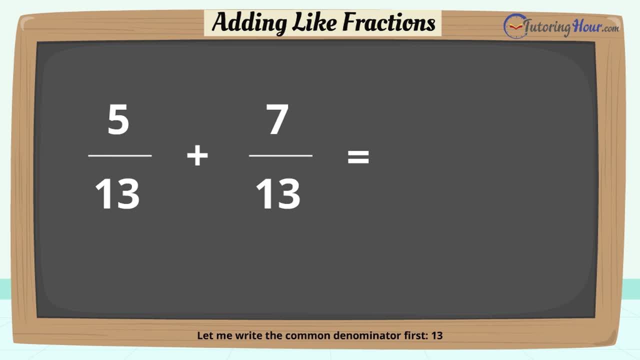 Let me write the common denominator first, 13.. Now I'll add the numerators 5 and 7 and write that as 5 plus 7 over the common denominator 13.. Adding them, I get 12 over 13.. Woohoo, That was quick. 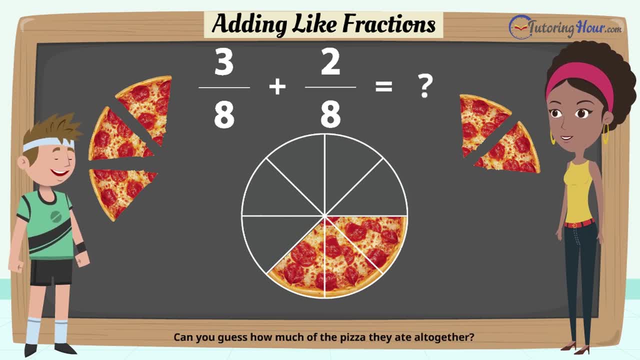 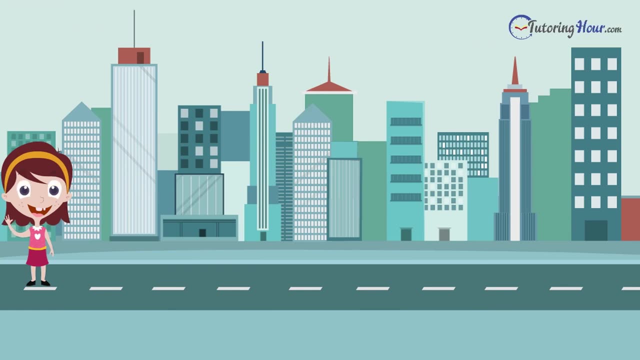 Can you guess how much of the pizza they ate altogether? Yes, you are right, Jake and Amanda ate five out of the eight slices, or five-eighths of the pizza altogether. Yippee, We've got the answer. Let's take another example. Linda walked four-ninths of a mile to reach the library and another three-ninths of a mile to reach the park. 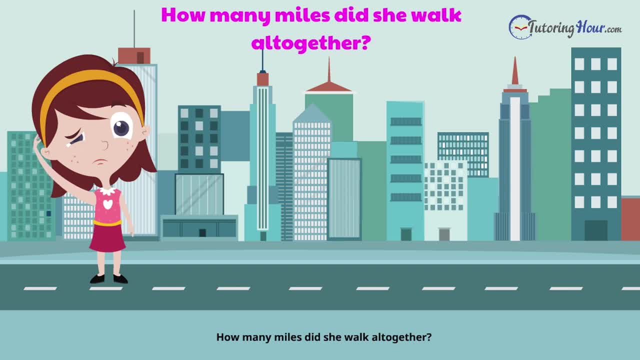 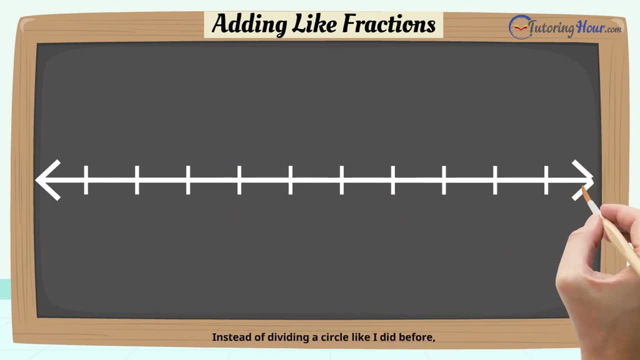 How many miles did she walk altogether? Let me show you an easy way to do it. This time I'll draw a number line. Instead of dividing a circle, like I did before, I'll divide the number line into nine equal parts between zero and one. 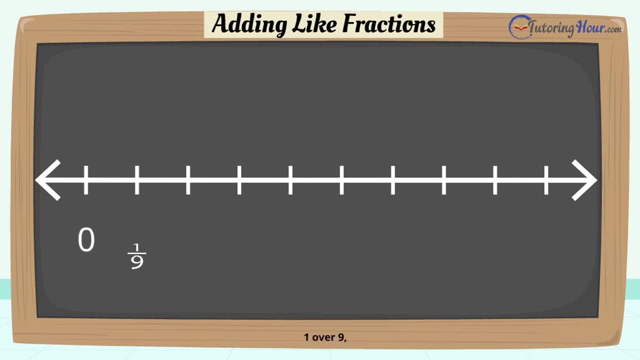 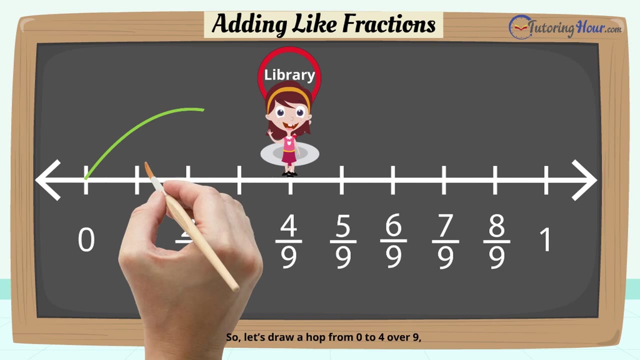 And I'll mark them zero, one over nine, two over nine, and go on until nine over nine, which becomes a whole. I'll write that as one. Now let's move on to the next step. Linda walked four-ninths of a mile, So let's draw a hop from zero to four over nine. 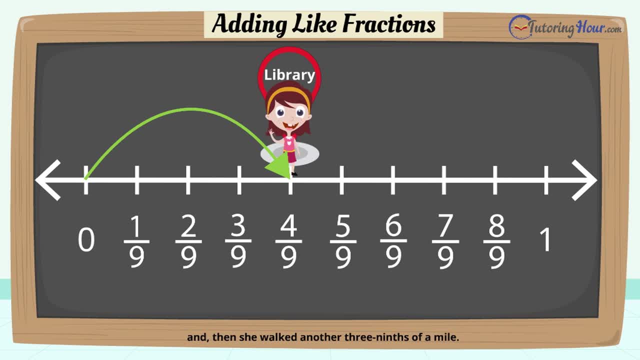 And then she walked another three-ninths of a mile, Starting at four over nine. I'll draw three more hops covering one-ninth, then two-ninths, and then two-ninths and then 3, 9ths of a mile, And that's it. Linda walked 7, 9ths of a mile in all. 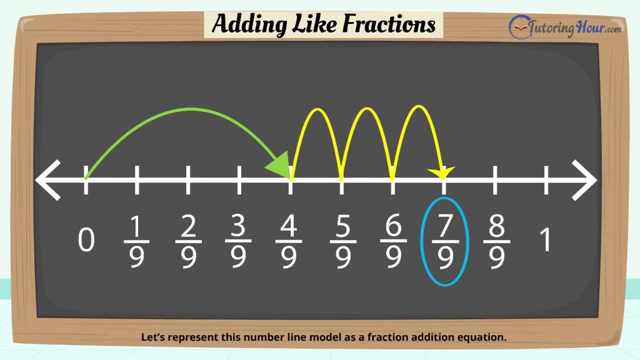 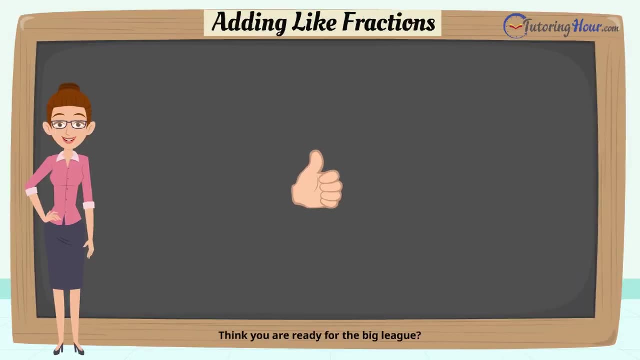 Let's represent this number line model as a fraction addition equation: 4 over 9 plus 3 over 9 makes 7 over 9.. Hooray, We have solved one more Great going. Thank you already for the big leak. 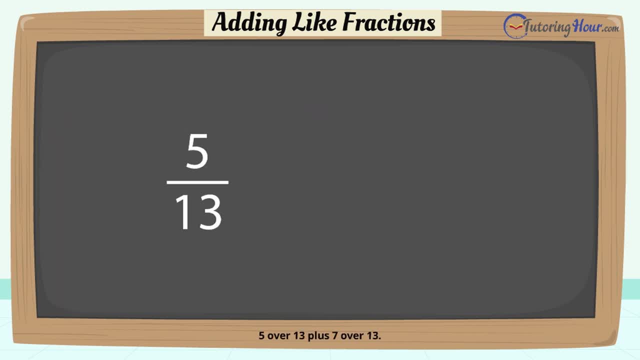 Then let's try another problem: 5 over 13 plus 7 over 13.. Look at both these fractions. They have the same denominators. When two fractions have the same denominators, we call them like fractions. While adding like fractions, we don't add the denominators, We simply retain them. 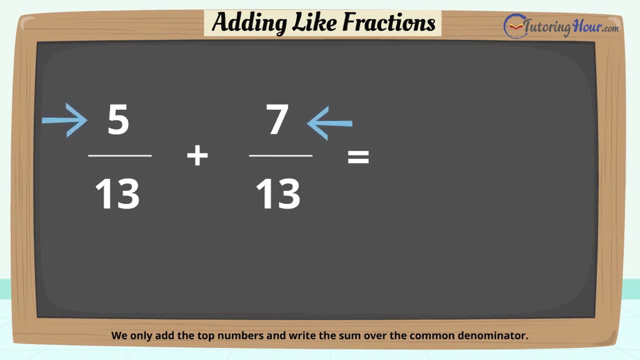 We only add the top numbers and write the sum over the common denominator. Let me write the common denominator first, 13.. Now I'll add the numerators 5 and 7 and write that as 5 plus 7 over the common denominator. 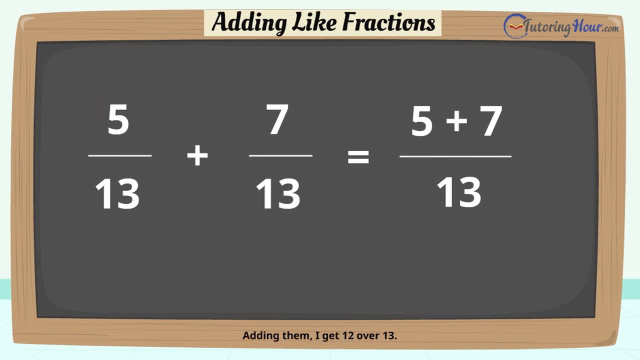 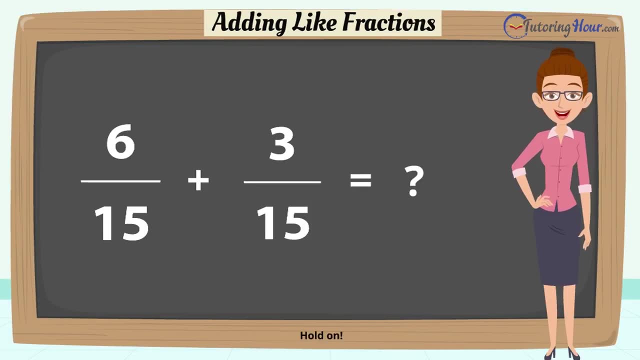 13.. Adding them, I get 12 over 13.. Woohoo, That was quick. Think you've mastered it. Hold on, This one may stump you because it has an added step. Let's work it out: 6 over 15 plus 3 over 15.. Both the fractions have the same denominators. 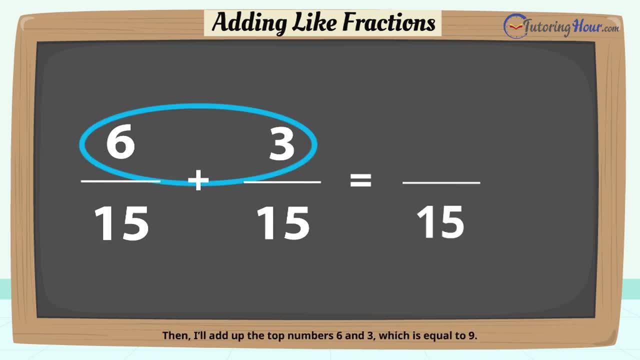 15.. I'll write that down. Then I'll add up the top numbers 6 and 3,, which is equal to 9.. The answer is 9 over 15.. And now comes the added step. Look at this fraction: 9 over 15.. 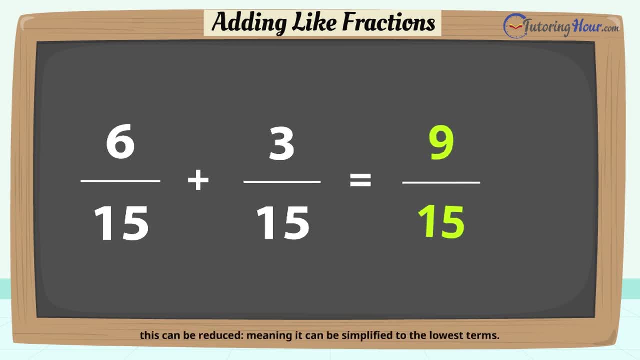 This can be reduced, meaning it can be simplified to the lowest terms. You may ask how? It's quite simple: Factor, the numerator and the denominator. 9 can be written as 3 times 3 and 15 can be written as 3.. 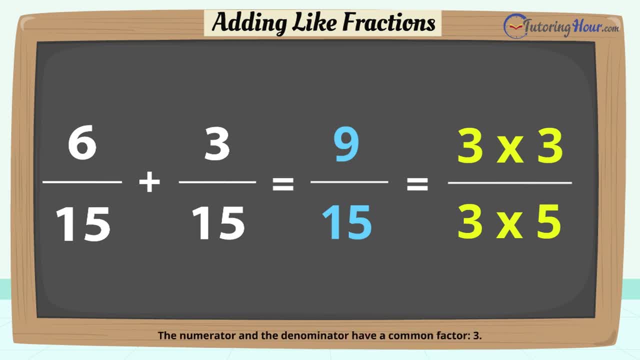 be written as 3 times 5.. The numerator and the denominator have a common factor: 3.. Let me circle that The 3 in the numerator and the 3 in the denominator cancel each other, leaving us with 3 over 5.. We understand that the fraction 9 over 15 simplifies to 3 over 5.. Now, that's a job well. 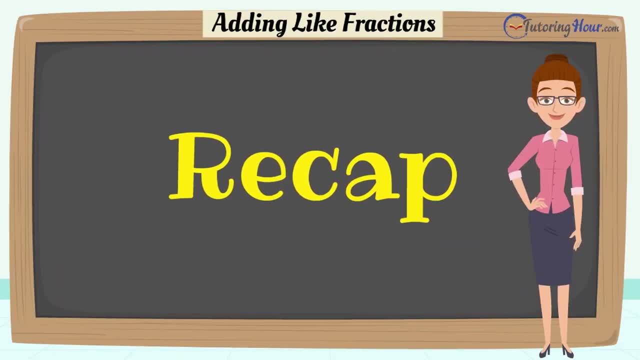 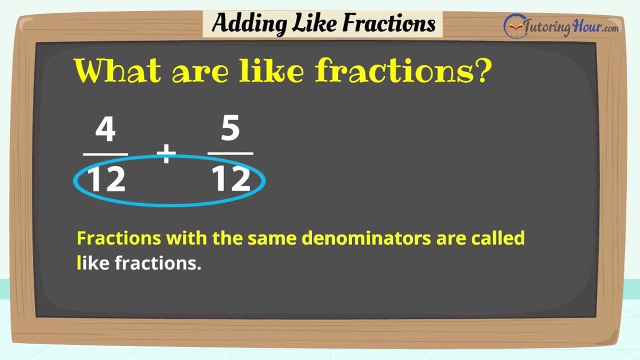 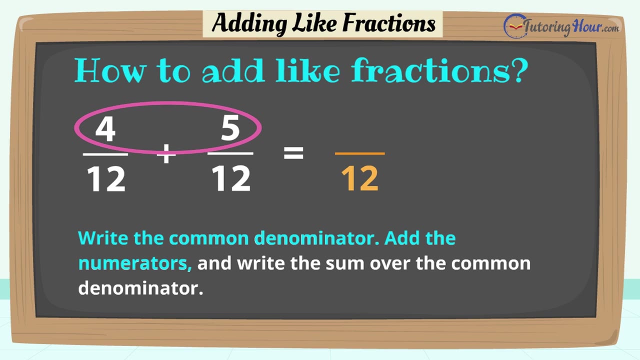 done. How about a quick recap? 1. What are like fractions? Fractions with the same denominators are called like fractions. 2. How to add like fractions, Write the common denominator, add the numerators and write the sum over the common denominator. 3. How to simplify or reduce. 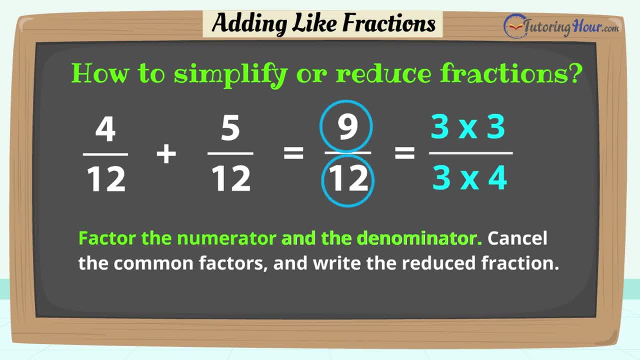 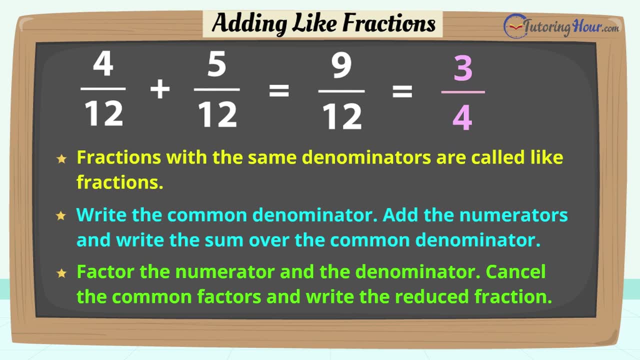 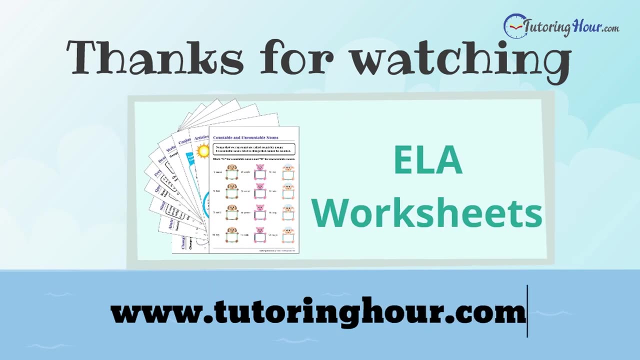 fractions, Factor the numerator and the denominator, cancel the common factors and write the denominator: reduced fraction. I strongly believe that practice makes perfect, and if you do too, then visit wwwtutoringhourcom, Check the link in the description box and download as many worksheets as you need and 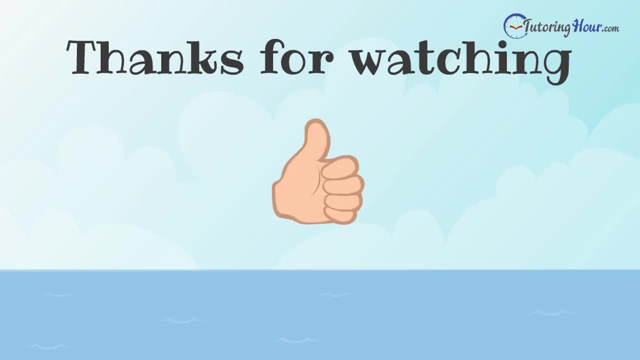 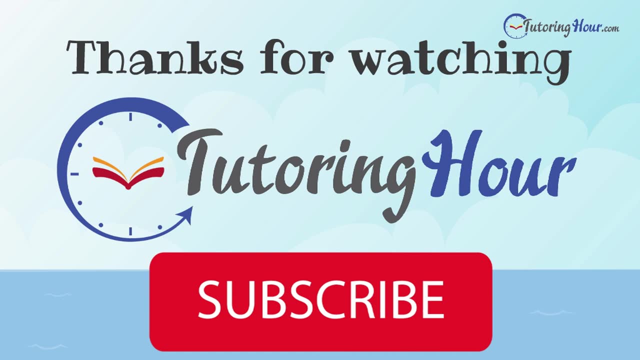 get practicing. If you liked the video, give us a thumbs up and don't forget to share the video with your friends, and remember to hit the subscribe button right now. Thanks for watching Tutoring Hour Subtitles by the Amaraorg community. 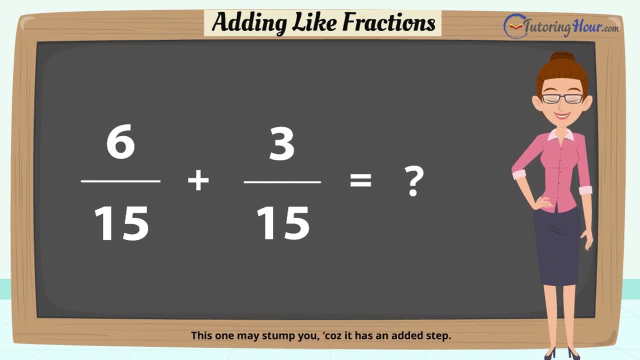 Think you've mastered it. Hold on. This one may stump you because it has an added step. Let's work it out: 6 over 15 plus 3 over 15.. Both the fractions have the same denominators: 15.. I'll write that down. Then I'll add up the top numbers, 6 and 3, which is equal to 9.. 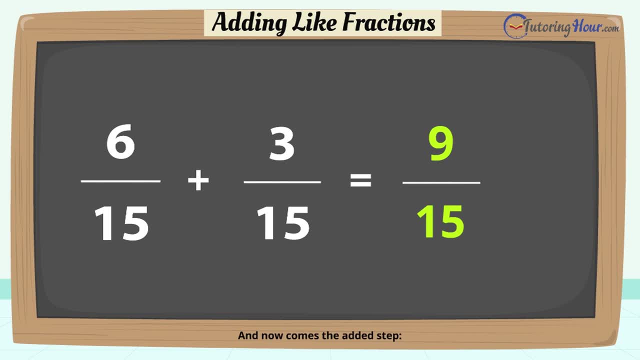 The answer is 9 over 15.. And now comes the added step. Look at this fraction: 9 over 15.. This can be reduced, meaning it can be simplified to the lowest terms. You may ask how? It's quite simple: Factor the numerator and the denominator. 9 can be written as 3 times 3, and 15 can be written as 3 times 3.. 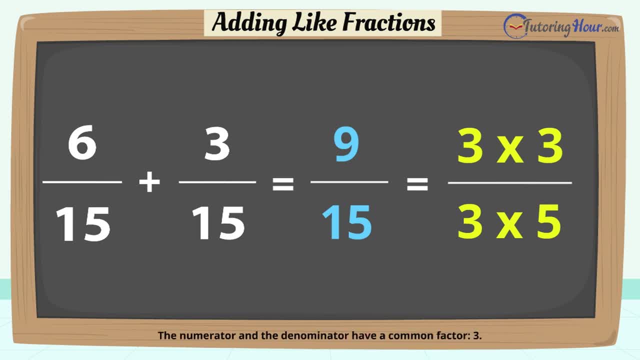 The numerator and the denominator have a common factor: 3.. Let me circle that The 3 in the numerator and the 3 in the denominator cancel each other, leaving us with 3 over 5.. We understand that the fraction 9 over 15 simplifies to 3 over 5.. Now, that's a job well done. 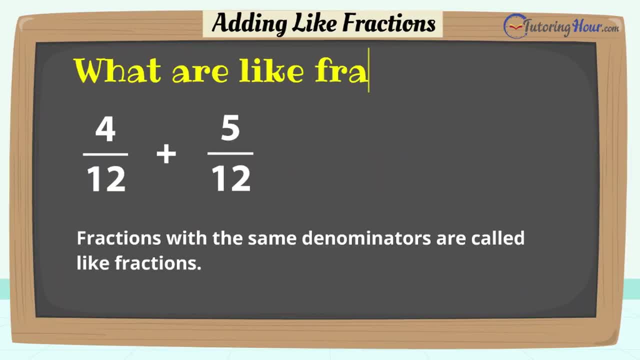 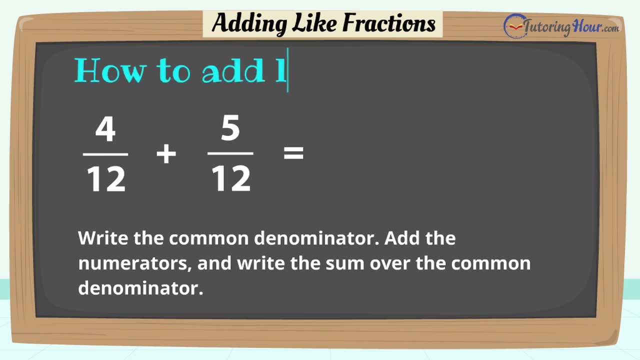 How about a quick recap? 1- What are like fractions? Fractions with the denominators are called like fractions. 2. How to add like fractions: Write the common denominator, add the numerators and write the sum over the common denominator. 3. How to simplify or reduce fractions: Factor the numerator and the. 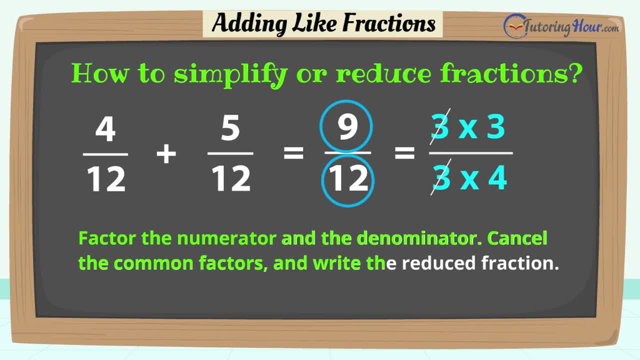 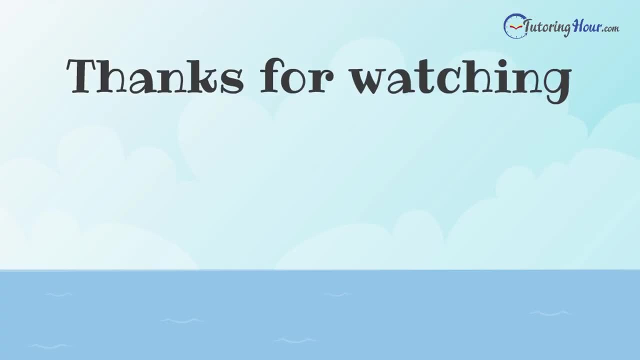 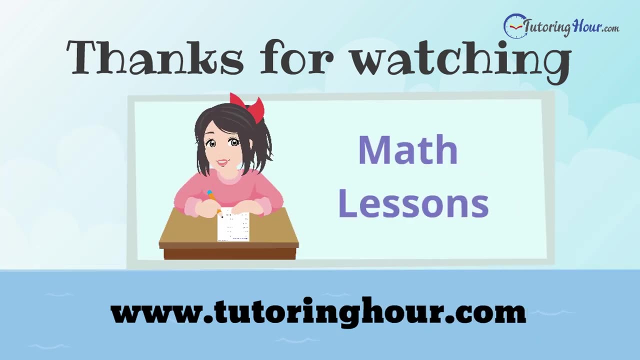 denominator, cancel the common factors and write the reduced fraction. I strongly believe that practice makes perfect, and if you do too, then visit wwwtutoringhourcom, Check the link in the description box and download as many worksheets as you need and get practicing. If you liked the video give: 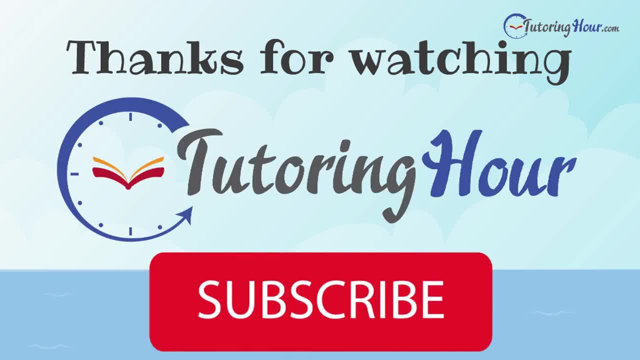 us a thumbs up and don't forget to share the video with your friends, and remember to hit the subscribe button right now. Thanks for watching Tutoring Hour.